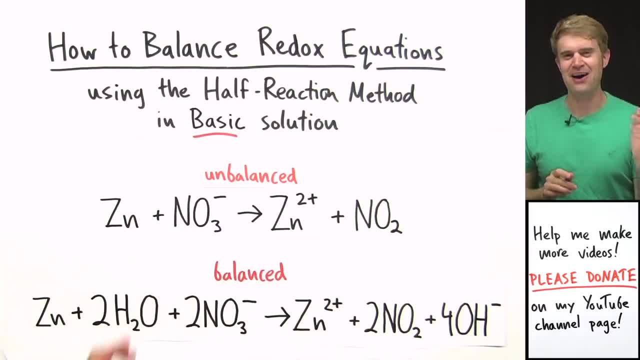 Now, if you're already a rock star at balancing redox equations in acidic solutions, feel free to skip through most of this video and just focus on the end part, where you'll see some extra steps used for balancing in basic solution that you don't use for balancing in acidic solution. 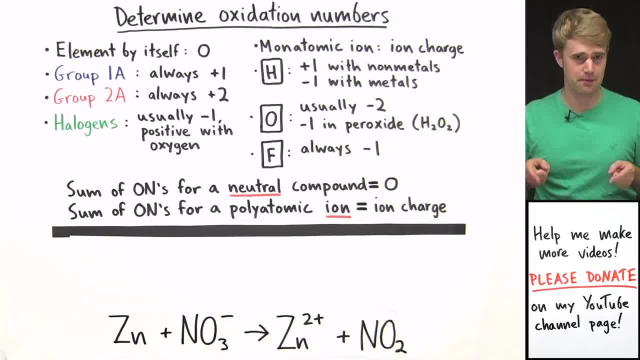 Got it, Let's get started. This is the equation that we're going to be balancing, and we're going to start just like we did in basic solution. So let's get started. We're going to start just like we do with acidic solution, by determining the oxidation. 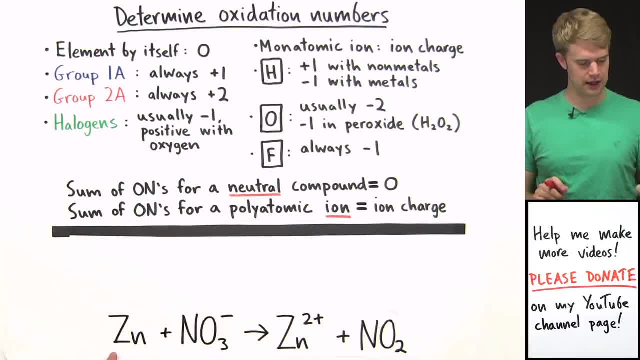 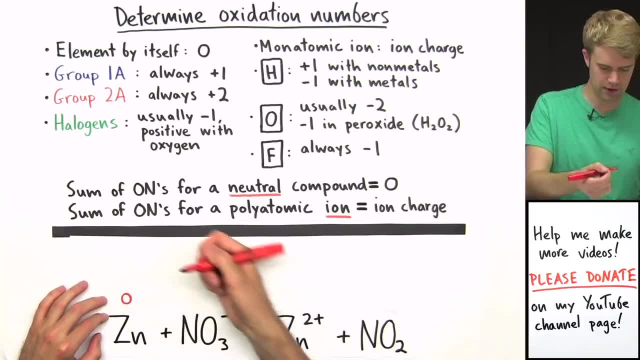 numbers of the elements in the equation. Okay, so starting here Zn. zinc is an element by itself. It's not combined with any other elements, so it has an oxidation number of zero. NO3- one minus- is a polyatomic ion. We don't know what nitrogen's oxidation number is, so we'll have 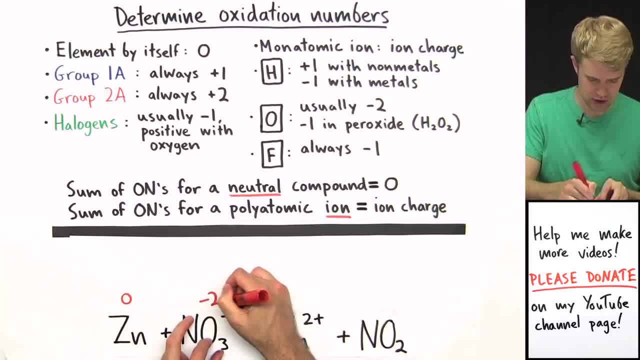 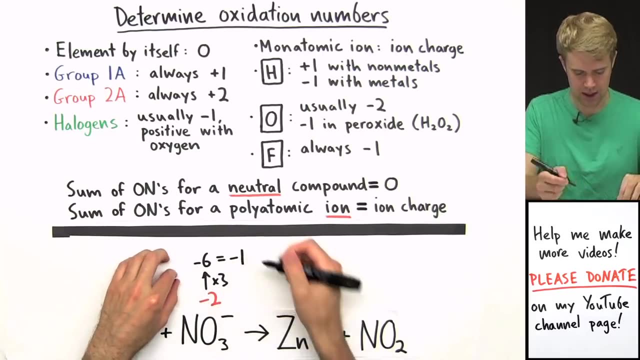 to figure it out, Oxygen is usually minus two. We have three oxygens here, so we'll do minus two times three. So we'll do minus two times three. Now, negative three gives us minus six. Now, whatever nitrogen's oxidation number is has to add with minus six to make minus one. 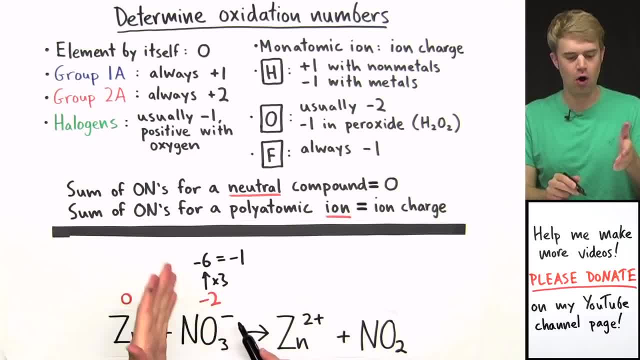 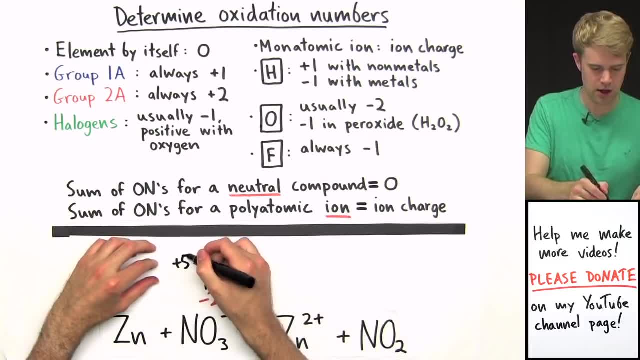 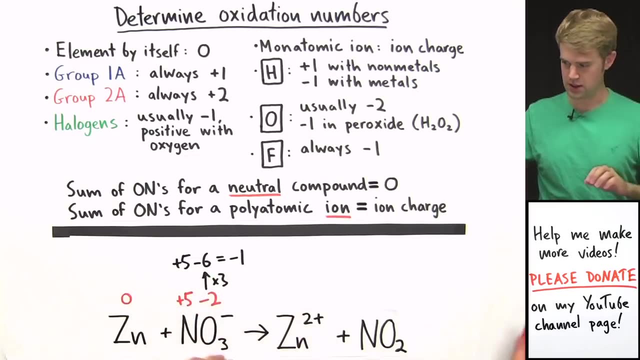 because that's a charge on this polyatomic ion and all of the oxidation numbers have to add up to this charge. So nitrogen's oxidation number is going to be plus five. plus five minus six equals minus one. so plus five for nitrogen over here on this side of the equation. 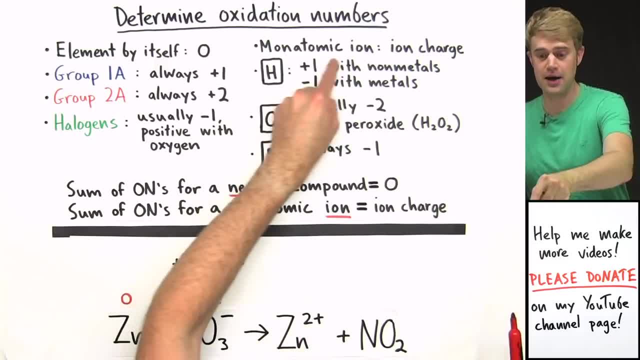 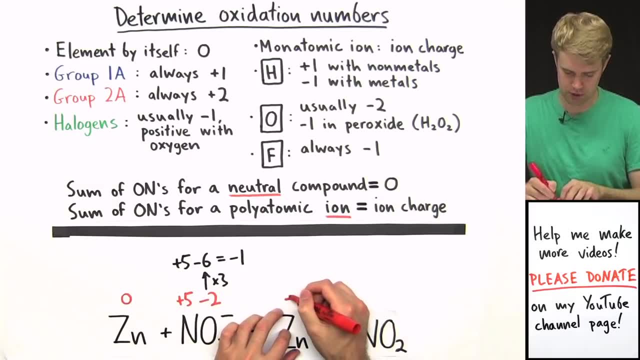 here on this side, zinc has become a monatomic ion with a charge of two plus, so its oxidation number is just gonna be the same as its ionic charge. okay, so plus two is zinc's oxidation number on this side. and then we got the same thing here with nitrogen. we got to figure out what it is. okay, oxygen is going to be minus two. we have two oxygens, so minus two times two gives us a total of minus four. no2: here is a neutral compound, though, so nitrogens and oxygens oxidation numbers are going to add to zero. so that means that nitrogens is going to be plus four, plus four, minus four. 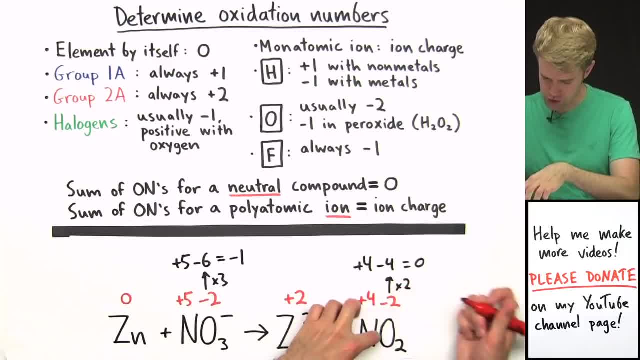 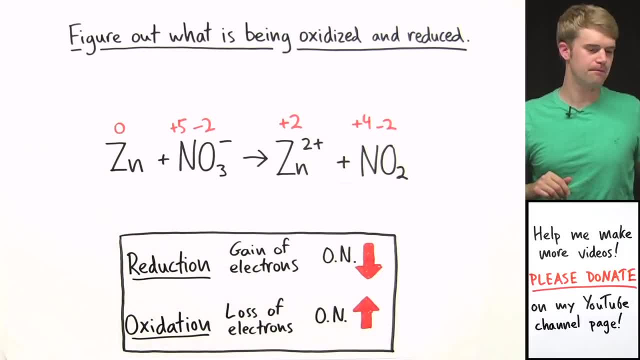 equals zero. so plus four for nitrogen on this side of the equation. so what's being oxidized and what's being reduced? we'll look at changes in oxidation number. okay, zinc here is zero on the left side of the equation and then it's plus two on the right side of the equation, so zinc's oxidation number is going up which? 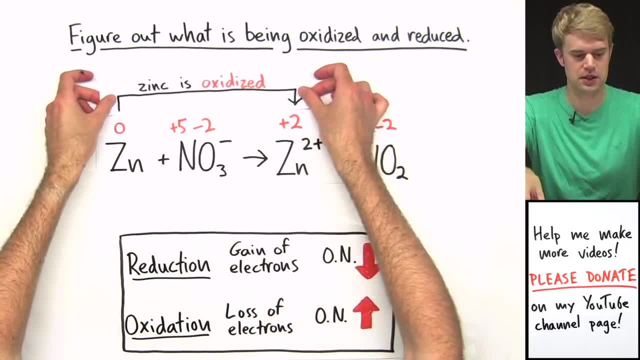 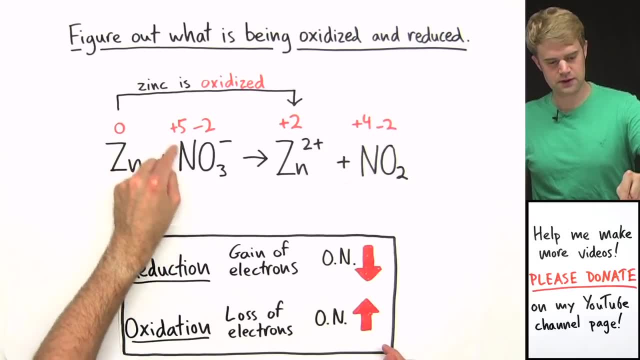 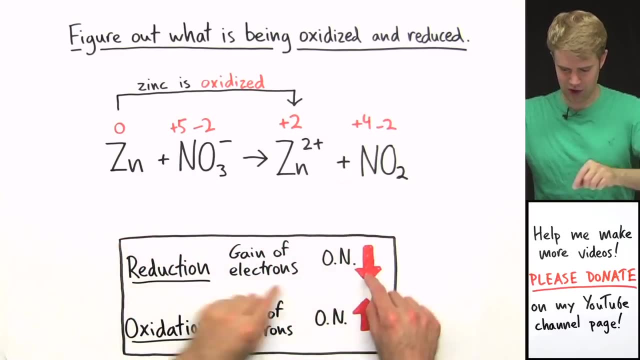 means that it is undergoing oxidation. so zinc here is oxidized from zero up to plus two. nitrogen here is plus five on this side and then it's plus four on this side. so its oxidation number is going down, it is undergoing reduction. nitrogen is getting reduced from plus five to plus four. 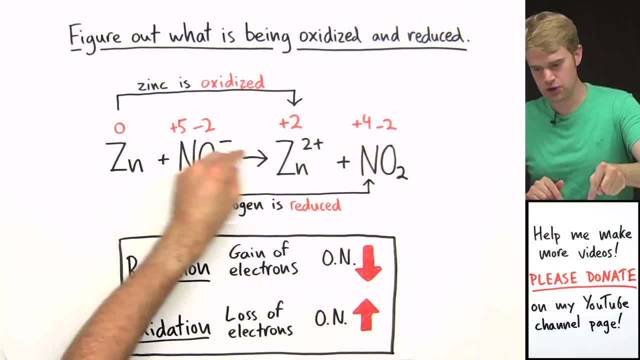 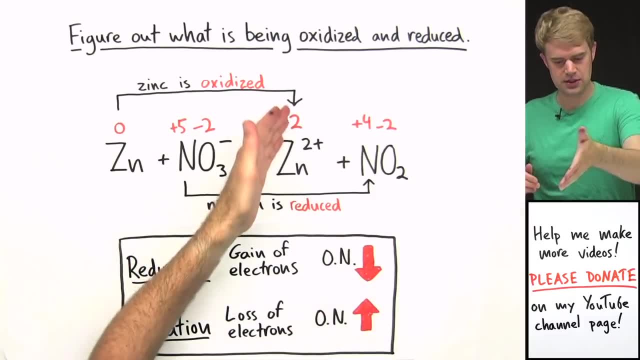 oxygen is on both sides of the equation. it's minus two here and minus two here, so it's neither oxidized nor reduced, so we don't have to worry about it at all. so zinc is oxidized, nitrogen is reduced. now let's write some half reactions for the oxidation. 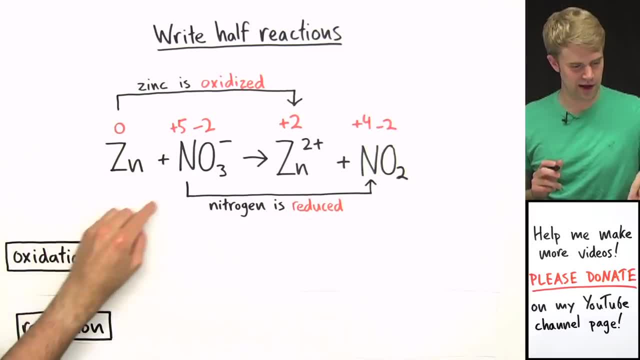 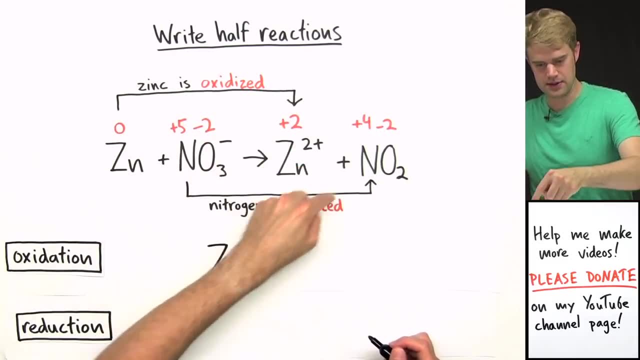 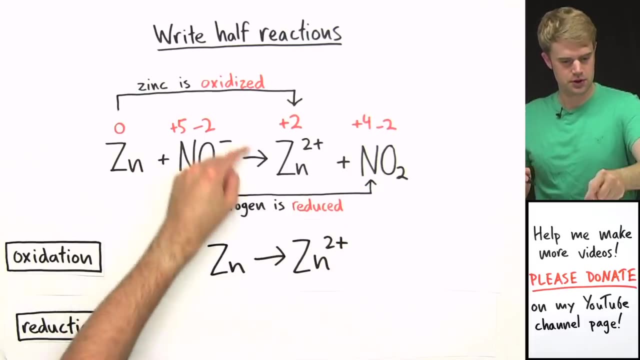 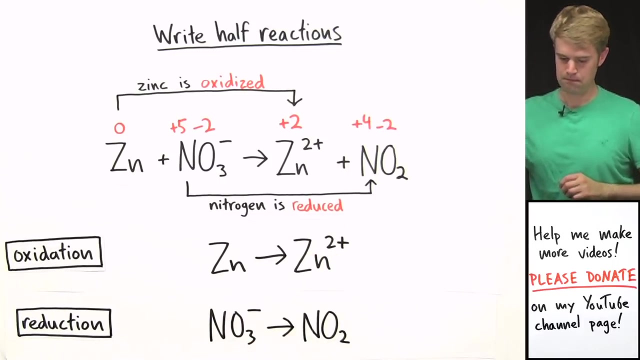 and the reduction. the oxidation half reaction is going to look like zinc, zn and then zn2 plus. on the right side nitrogen is getting reduced. so on the left side of the reduction, half reaction is going to be n o three, one minus. then we got the arrow, and then the right side, n o two. okay, now let's balance each. 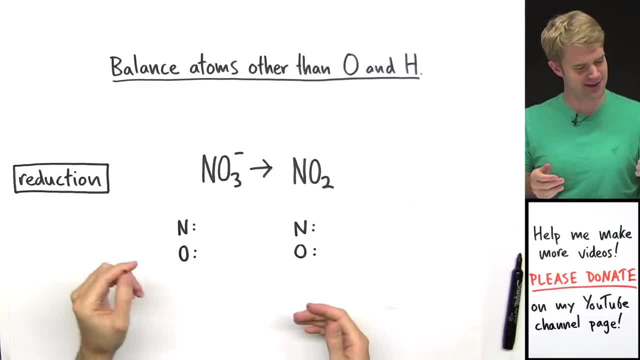 one of these. we'll start by balancing the reduction half reaction. what's this on my uh got some marker on the finger. it's an occupational hazard. sometimes i'll go out with my friends in the evenings and they'll be like: you're doing a video today, right, and i'll be like, how did you know? and it's because my hands are just 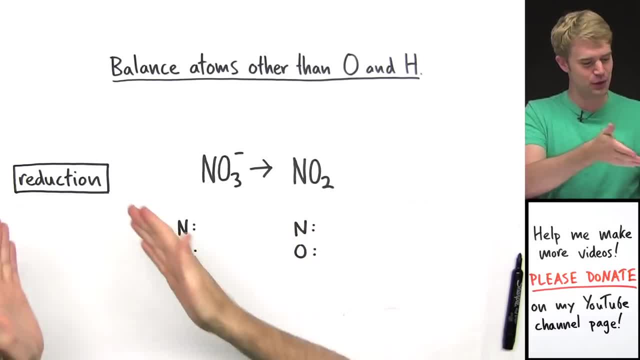 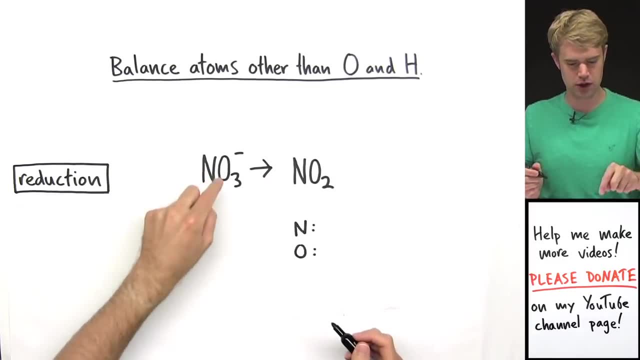 covered with marker. anyway, we're going to balance the reduction half reaction. we have two elements right now: nitrogen and oxygen. okay, so on this side we have one nitrogen, we have o3, we have three oxygens. then on this side, we have one nitrogen and we have o2, we have two oxygens. 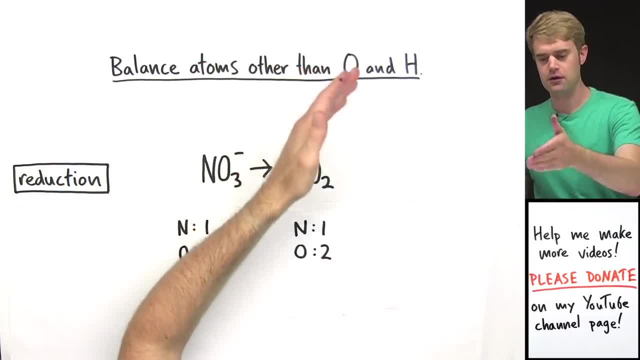 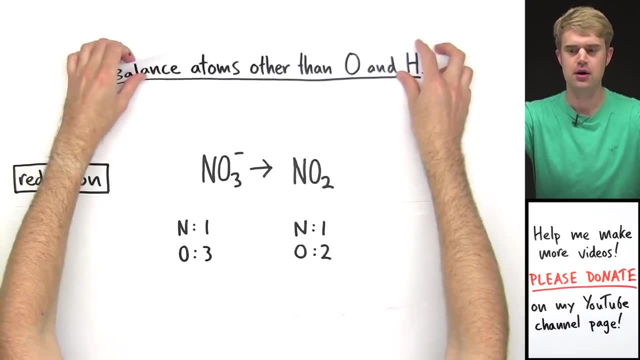 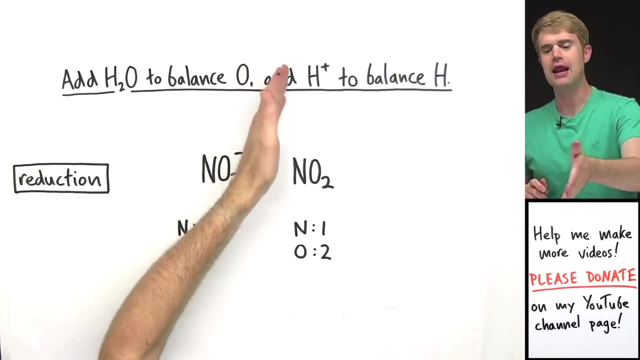 so our first step is to balance the atoms other than oxygen and hydrogen. that would be nitrogen here, and we're all set. we have one nitrogen on this side and one nitrogen on this side, so let's move on to the, the next step here. add h2o to balance o and h plus to balance h. okay, so right now, let's focus in on oxygen. there is an. 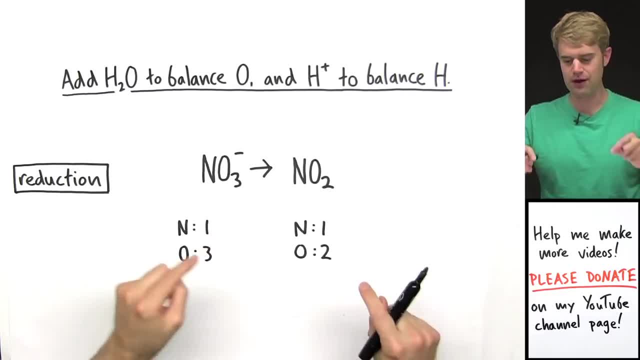 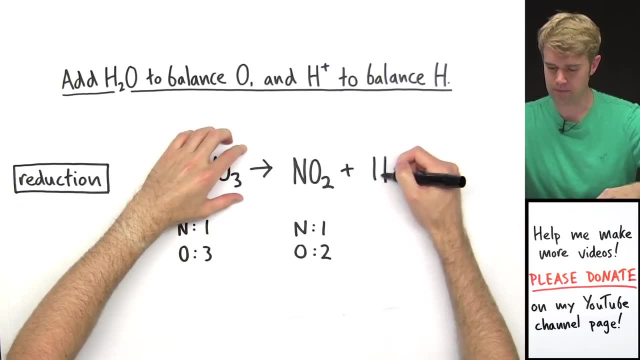 imbalance in the number of oxygens. we have three on this side and we have two on this side, so i need to add more oxygens to this side. okay, so i'm going to add h2o here now. how many h2os do i want? 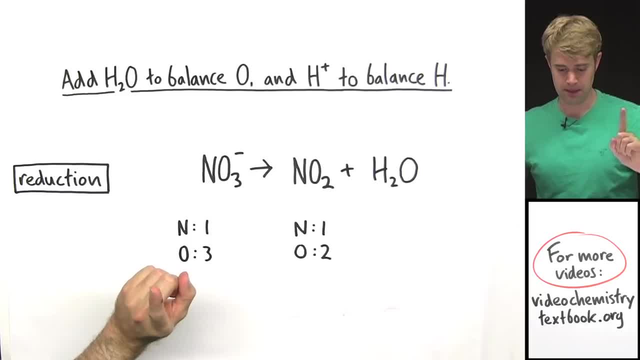 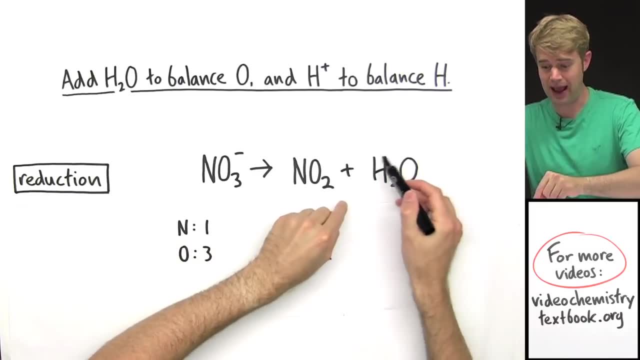 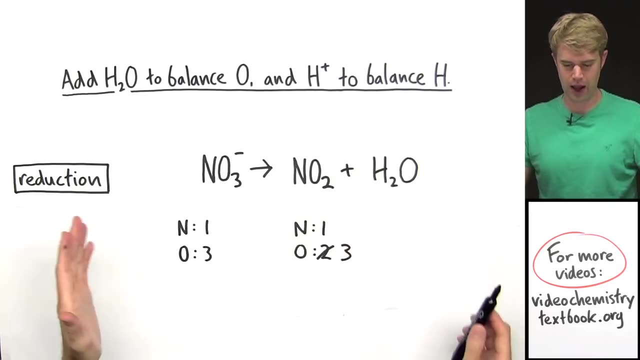 each h2o molecule has one oxygen atom. i have two, i need three so they balance. so all i need is one oxygen atom. okay, so by adding just one h2o i get that one oxygen i need. so i can go from two to three on this side. okay, all set nitrogens and oxygens balance, but by adding this h2o i introduced. 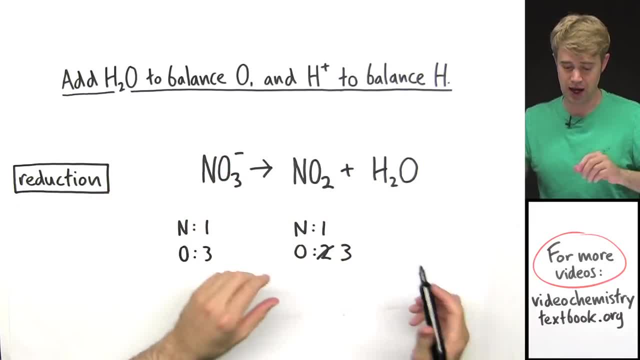 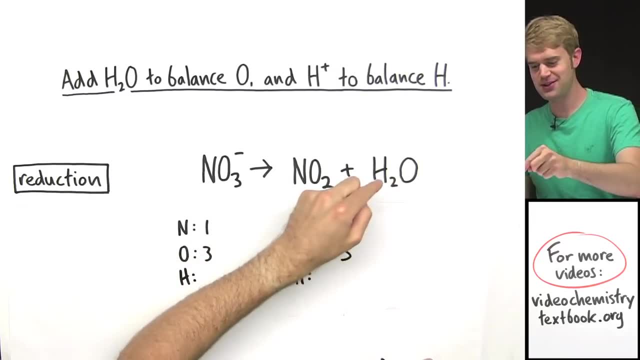 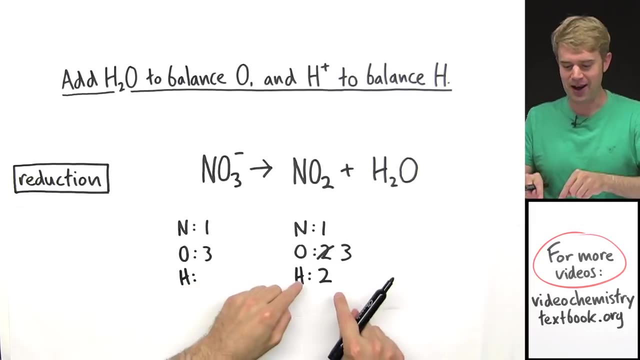 a new element into the equation and that's hydrogen. okay, so now we gotta- now we gotta put that in this equation in here. okay, h2- there are two hydrogens in h2o, so I got two on this side. right now, I have zero on this side, okay, so that's a problem, but I can balance out. 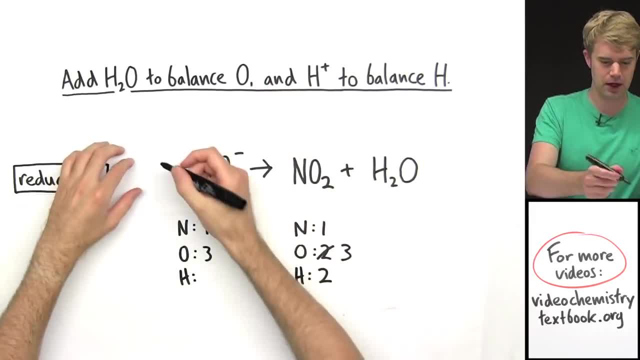 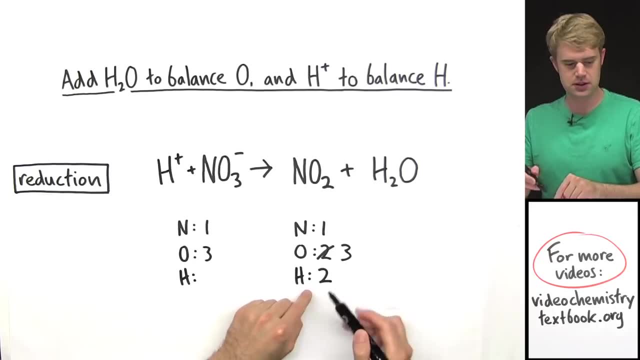 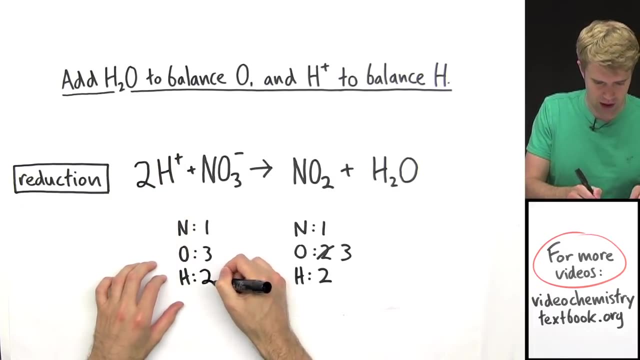 my hydrogens by adding H plus. okay, so here's my H plus. how many H pluses do I need? I have two hydrogens on this side, so I'm gonna make two H pluses on this side. so now, that's gonna give me two hydrogens here on the left. now real. 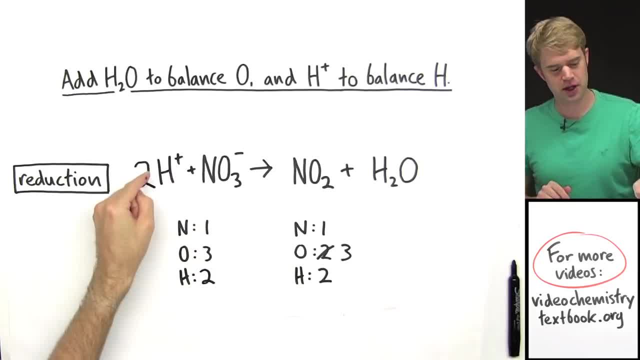 quick about these H pluses. adding H pluses to something makes it more acidic. we're supposed to be balancing this equation in basic solution, but we're gonna worry about the basic part later. okay, so right now we add the H pluses. they temporarily make it acidic, but then in some of the end steps we add: 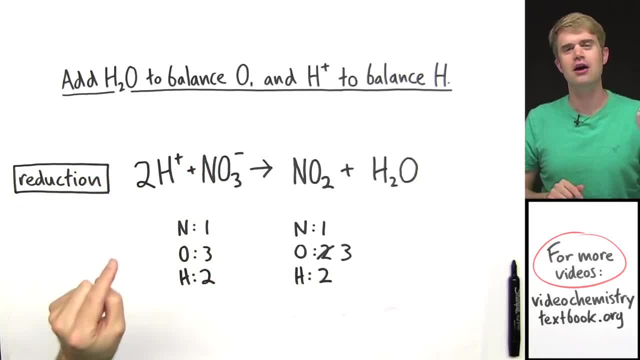 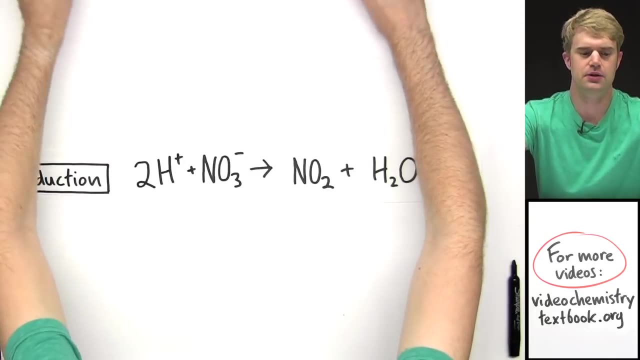 additional OH minuses to cancel out the H pluses. so don't worry about this for right now, even though it does make the equation acidic. okay. so the atoms all balance nitrogen, oxygen and hydrogen. the last thing we want to do for the reduction half reaction here is to balance the 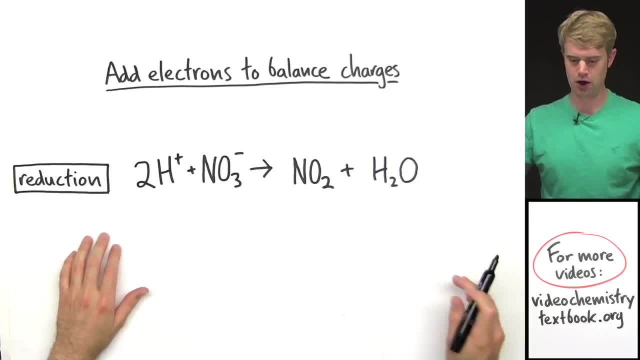 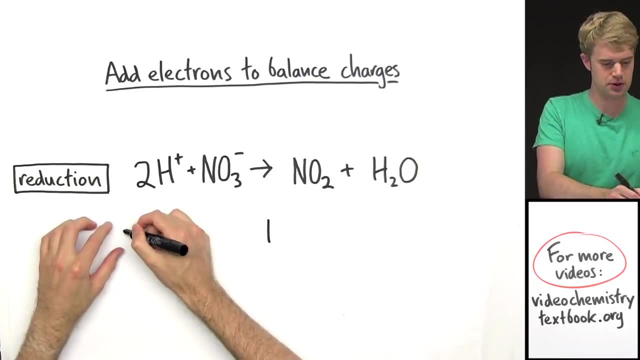 charges by adding electrons. so let's take a look at the charge situation in the equation. okay, on the left side we have 2 H plus, so that's going to be plus 2, and then we have 1 NO3, 1 minus, so that's going to be plus 2, and then we have 1 NO3, 1 minus. 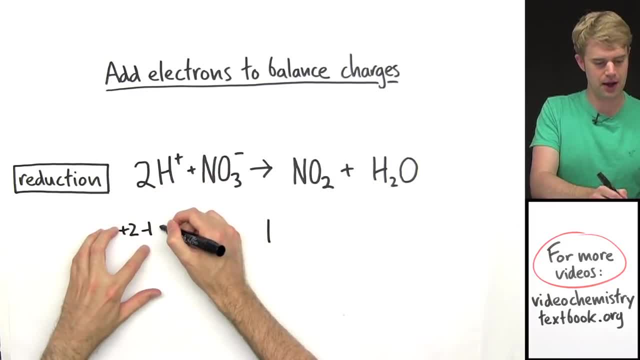 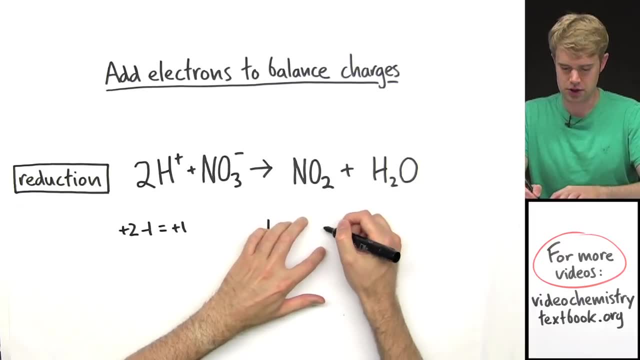 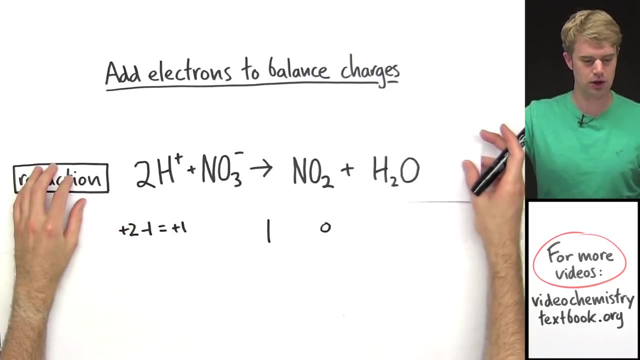 that's going to be minus 1 plus 2. minus 1 equals plus 1. and then here on the right side, we don't have anything that's charged, so we just have a charge of 0. okay, so what I need to do in order to balance these is to lower the charge on. 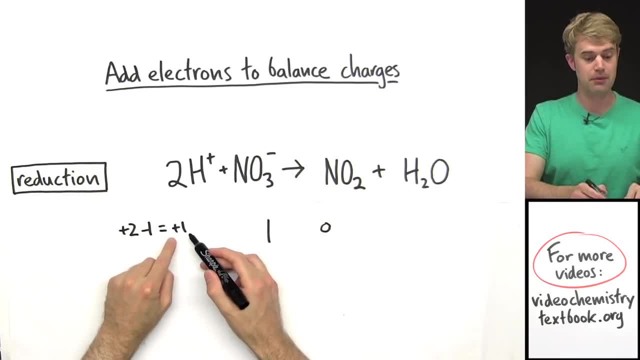 the the left side here and I can do that by adding one electron here. it is E minus. this electron has one negative charge. so adding to the left side plus 1 minus 1 for that one electron gives me 0. now I got 0 on this side. let's line that up now. I got 0 on this side and I got 0 on. 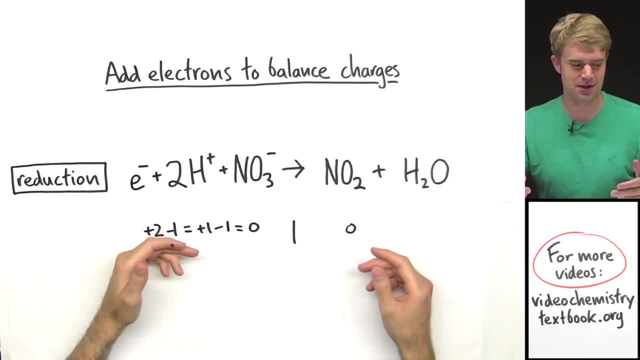 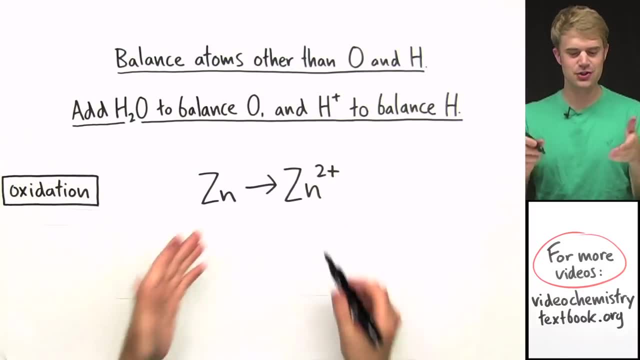 this side. the charges are balanced, the atoms are balanced, and now I'm going to move on and balance atoms and charges for the oxidation half reaction. balancing the atoms for the oxidation half reaction is going to be pretty easy, because all I have is one element here and I have one atom of each on both. 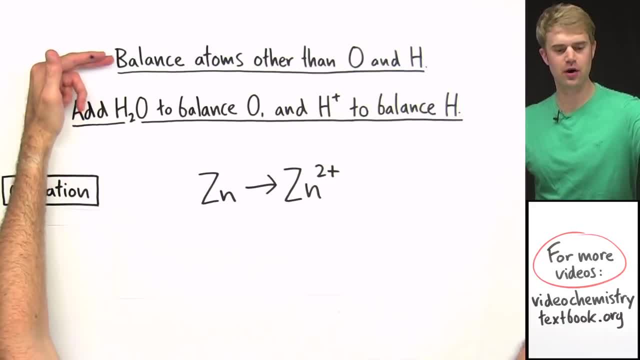 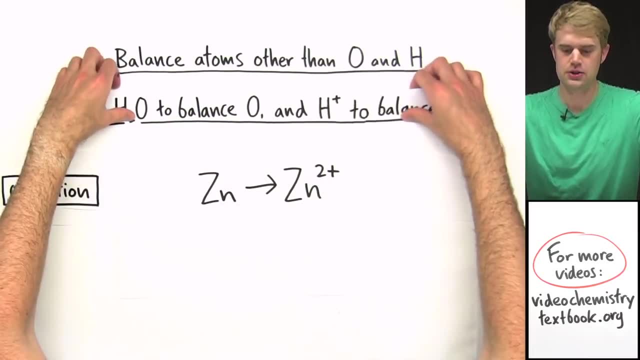 sides: one zinc here, one zinc here. so I don't have to worry about balancing the atoms other than oxygen and hydrogen. and I don't have to do any of this stuff with oxygen and hydrogen because I don't have those, so I can skip right ahead to. 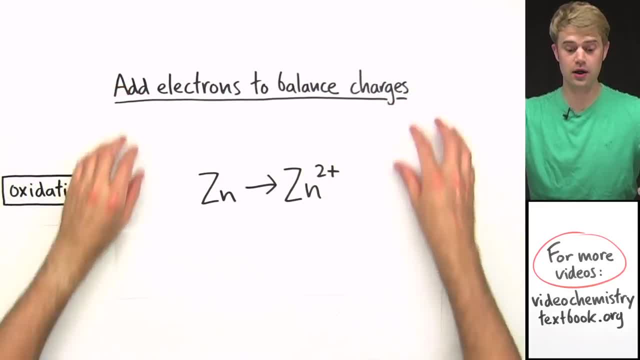 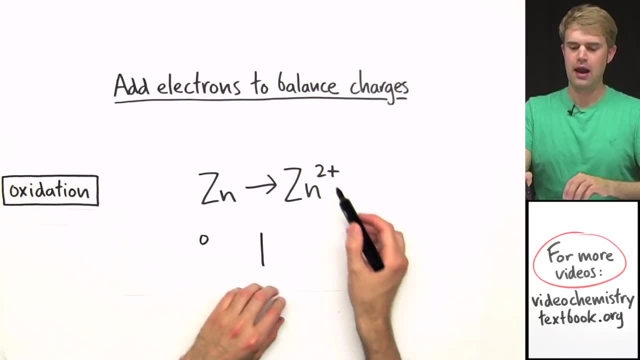 adding electrons to balance the charges. we are gonna have to do this. let's take a look at the charge here. on this side I don't have anything that's charged, so I have 0 charge, and then over here I have 1 ZN 2 plus, so I have plus 2 of charge. 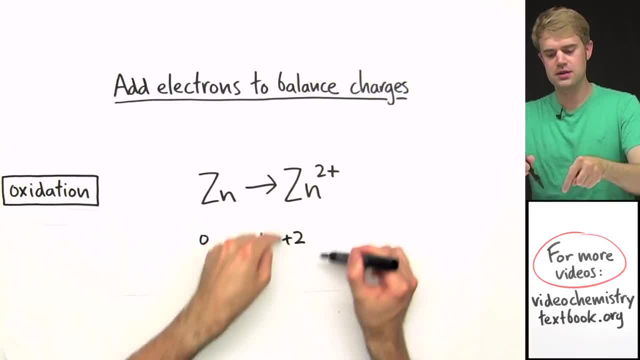 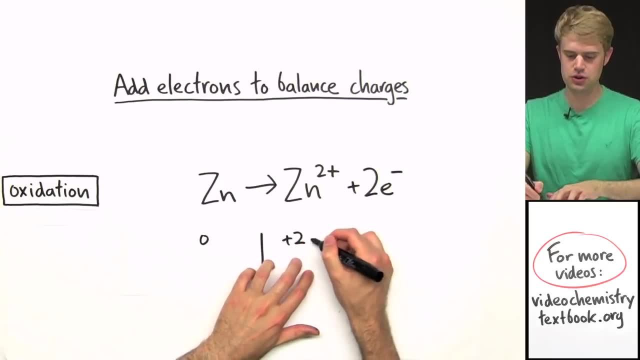 here. in order to get these to balance, I'm going to have to do a little bit of a balance. I got to lower this side by 2, so I'm going to add 2 e minus 2 electrons that have a negative charge, so I'm gonna have plus 2. minus 2 gives me 0. now I got. 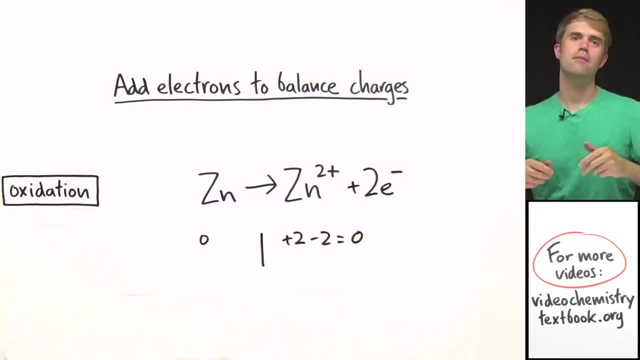 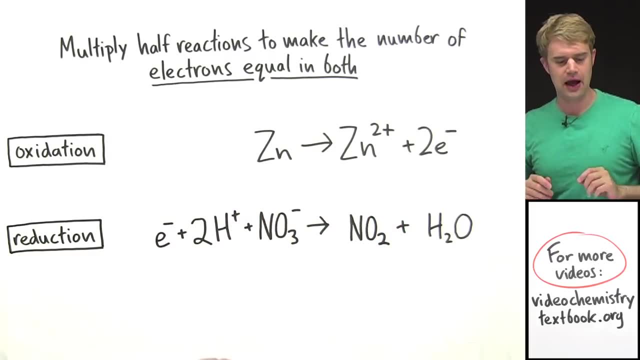 0 charge on both sides and these charges balance. now I'm going to start to put the oxidation and reduction half reactions together, but in order to do that I've got to have the same number of electrons in both of them, and right now I don't have that. I've got two electrons up here and I have 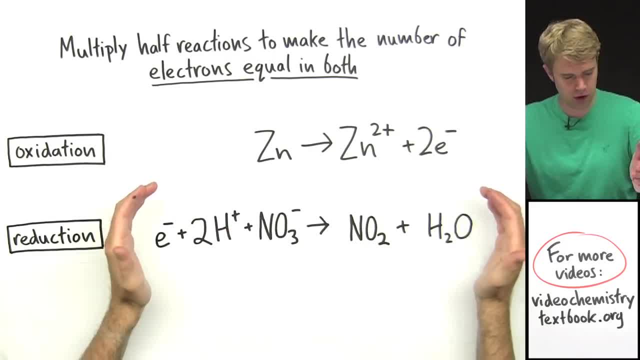 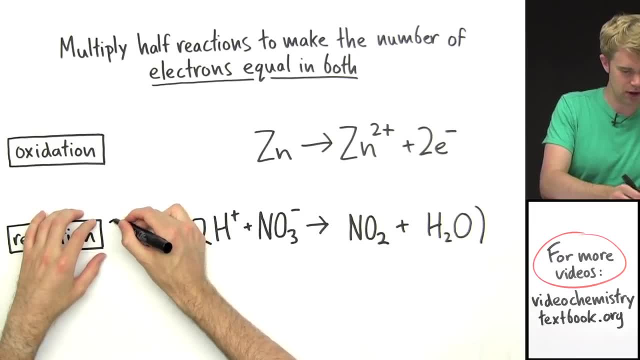 one electron down here. so to change that, I'm gonna multiply this whole reduction half reaction by 2, just kind of like it's a. it's a math equation, okay. so now I've got 2 times all of this. I'm gonna distribute the 2 across this reaction. 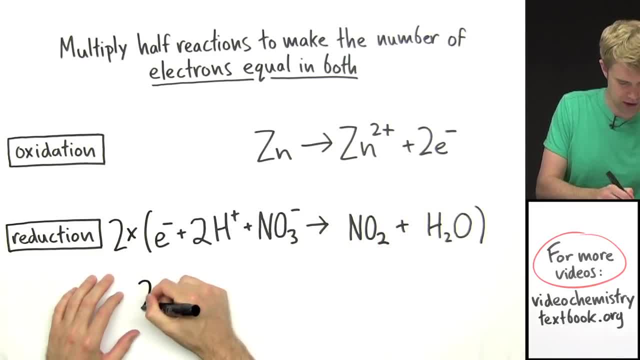 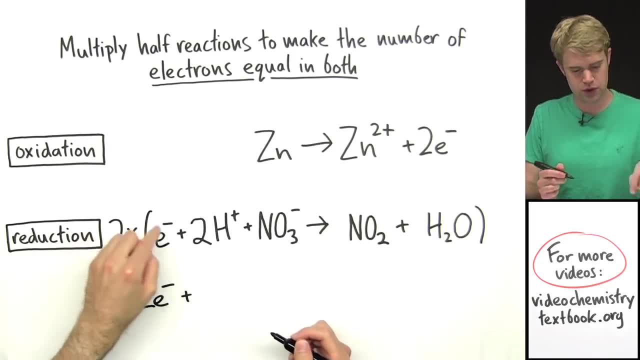 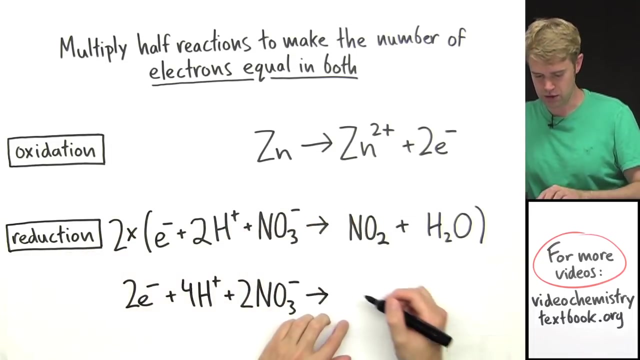 okay, so 2 times e minus is gonna give me 2 electrons. perfect, now the electrons are the same in both. okay, 2 electrons plus 2 times 2 H plus is gonna be 4 H plus plus 2 times that is 2 NO3, 1 minus. then we got the arrow 2 times NO2, 2 NO2 plus. 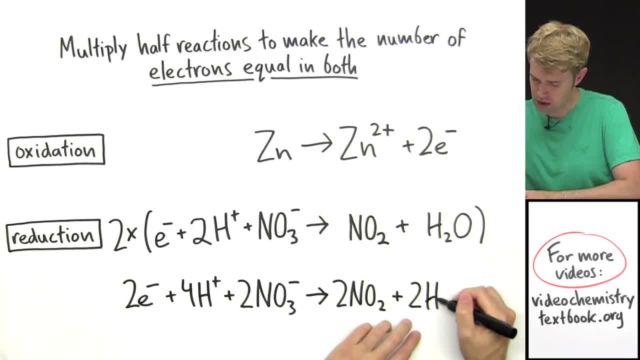 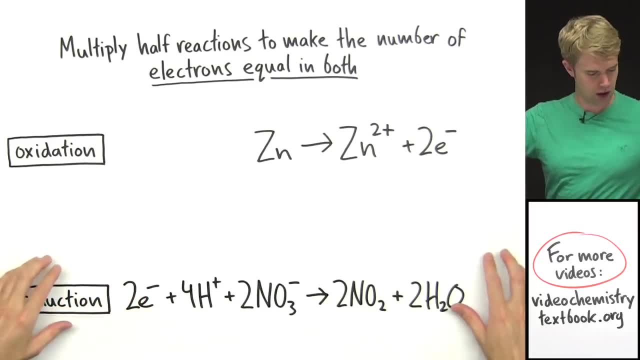 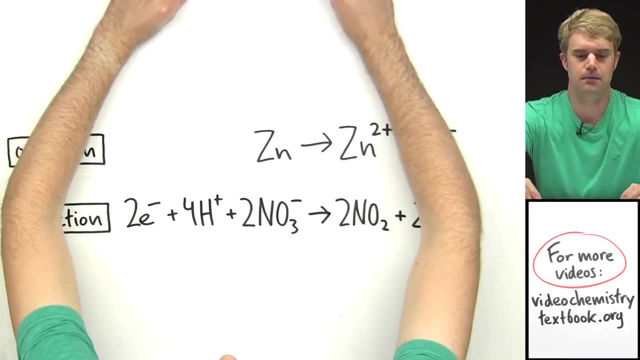 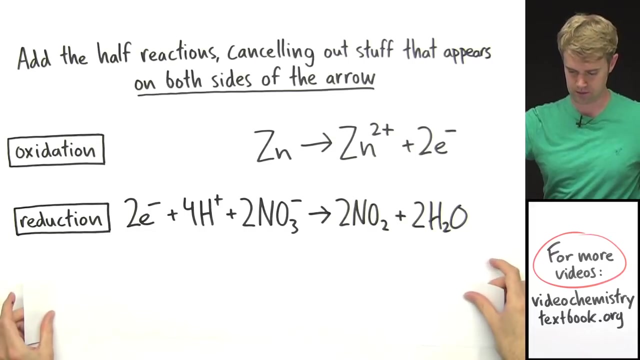 2 times H2O, 2 H2O. okay, so now the electrons are equal and this is my new reduction, half reaction. so now that I have the same number of electrons, I can add them together. I'll add them together and then cancel stuff out that appears on both sides of the arrow, so let's do that to. 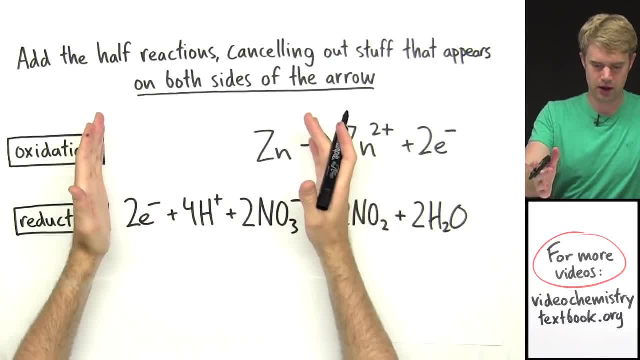 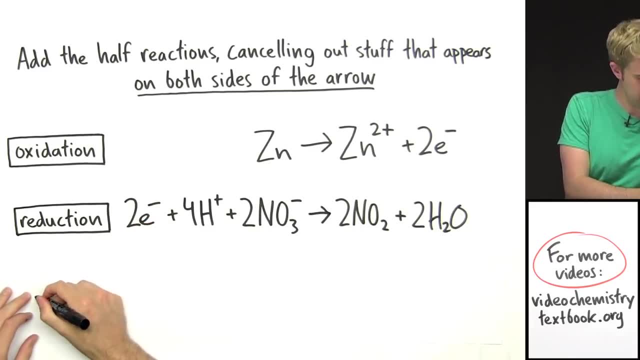 add these together. I look at the arrow and I choose everything from both equations on the left side of that to start with. okay, so left side, we start with ZN, ZN. and now I move down here for everything to the left of the arrow in this reaction: ZN plus 2 e minus. 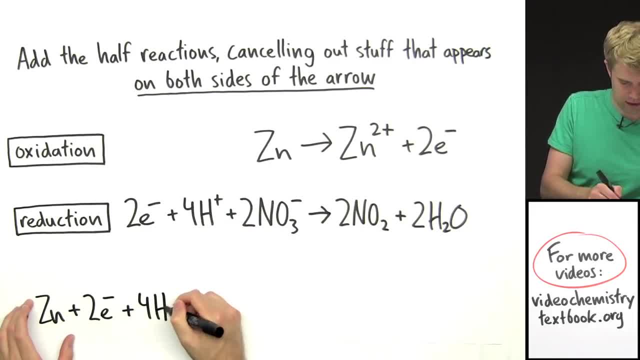 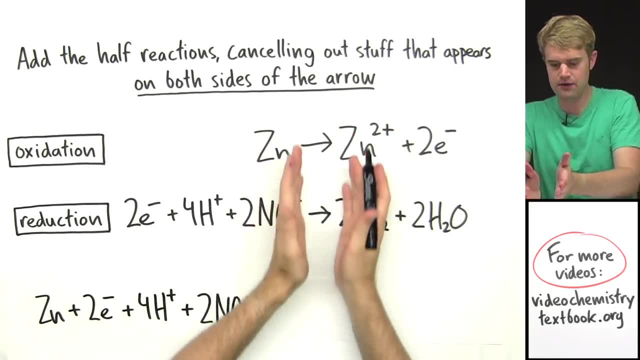 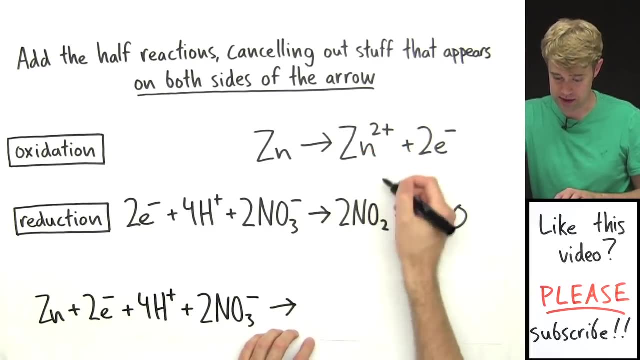 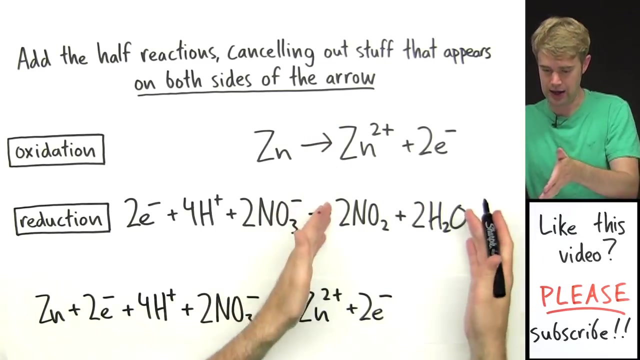 plus 4, H plus plus 2, NO3, 1 minus. then I have the arrow in both of them. so I put the arrow here and now everything on the right side of the arrow for both the equations. so I have ZN 2 plus, ZN 2 plus plus 2 e minus, and now down to here, plus 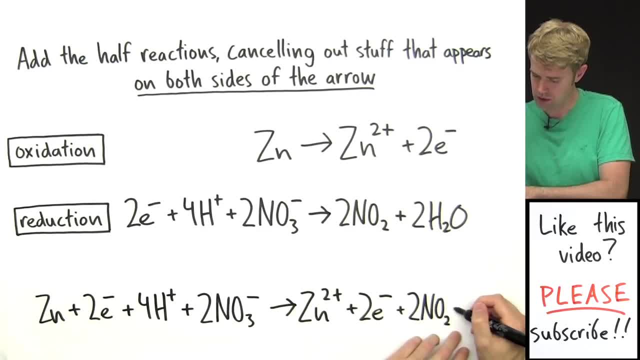 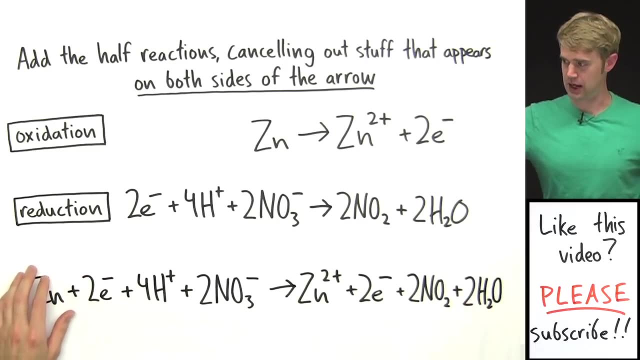 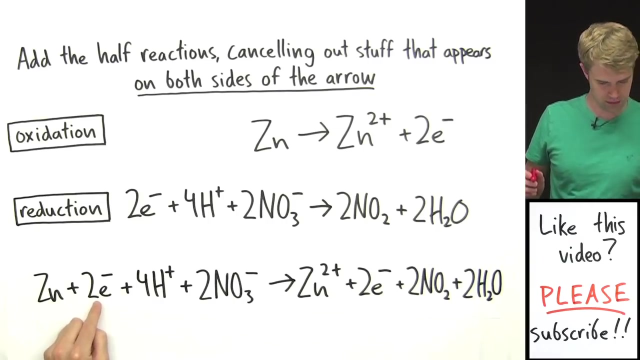 2 NO2 plus finally, 2 H2O- a little bit of a tight squeeze- plus 2 H2O. okay, now what I want to do is I want to cancel out stuff that appears on both sides of the arrow and for this equation here, that is, these two electrons, 2 e minus. here, 2 e minus. 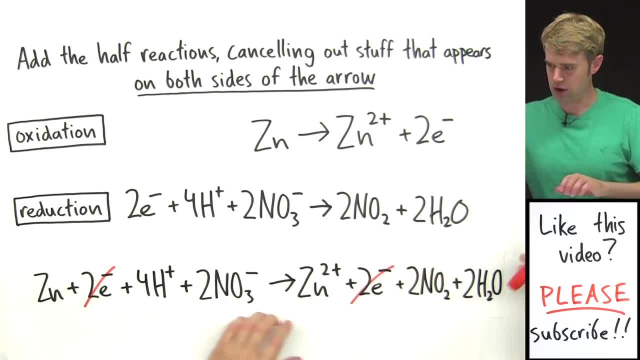 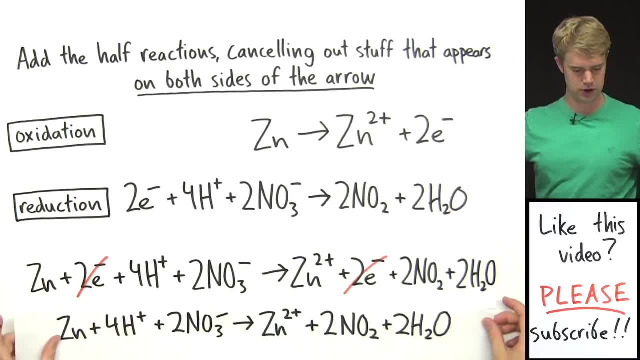 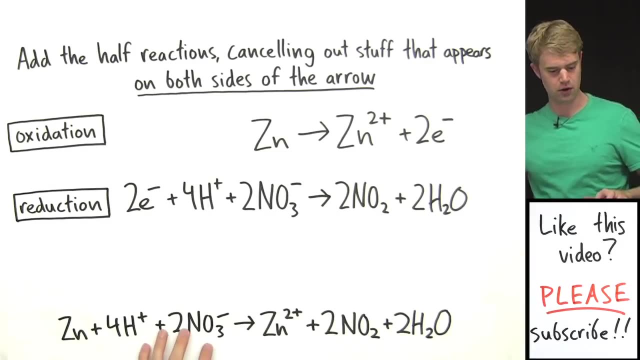 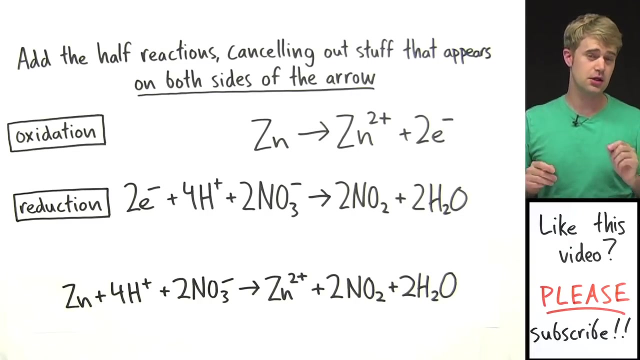 here, okay, so get rid of those, get rid of those. and now, when I rewrite this, to get rid of the electrons. the equation is going to look like this: just the same thing with everything else, except for the electrons. so there it is for you now. if our goal was to balance this in acidic solution, we'd be all set. 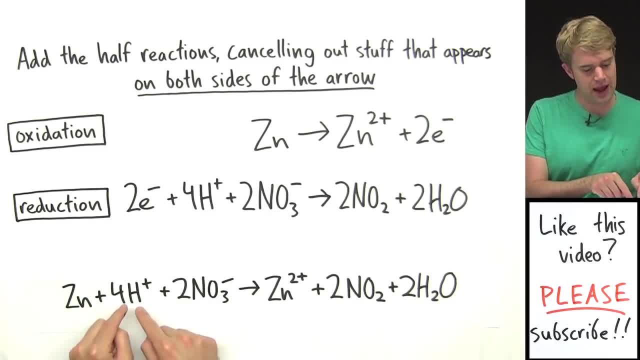 everything balances now and we're left with H pluses here, which make the equation acidic. but we've got to balance this in basic solution, which means we're gonna have to go through a couple more steps to get rid of these H pluses and replace them with OH minuses, which make things basic. so let's start to. 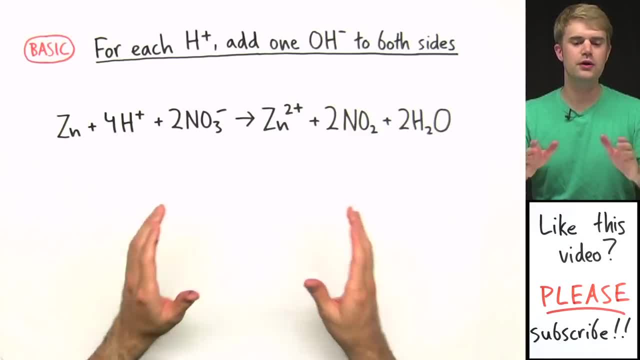 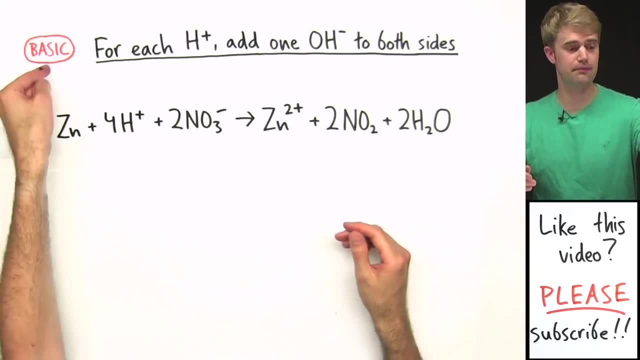 turn this into a basic equation. here's the first step that we use only for balancing in basic solution. that's why I put this little basic above here. this is an extra step at the end if you're balancing in basic solution. okay, as I said, we got to get rid of these H pluses because the H pluses makes something. 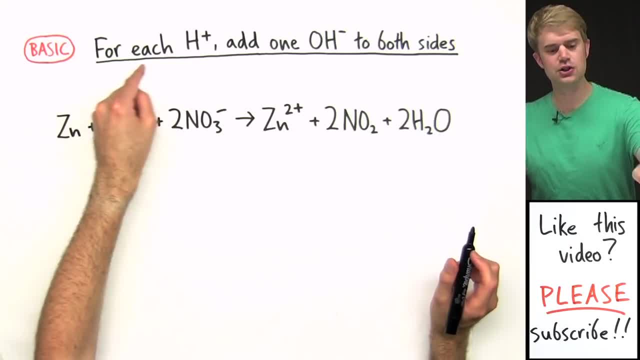 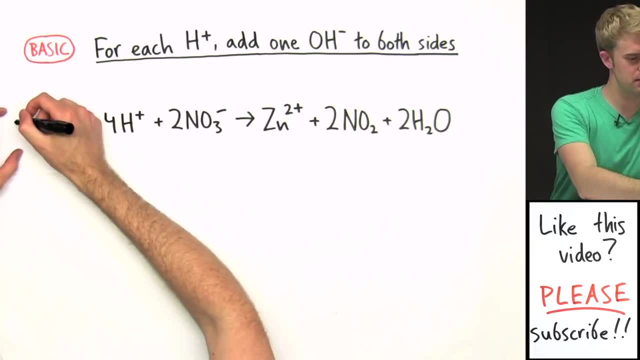 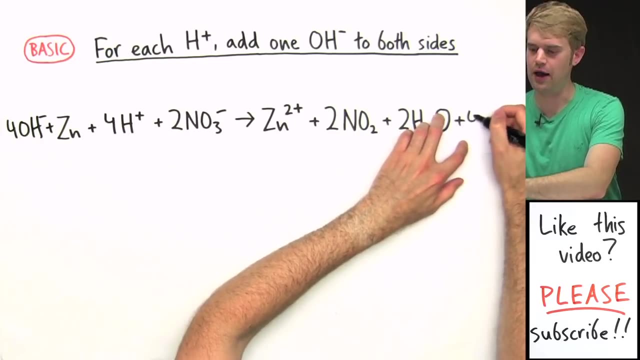 acidic. so to get rid of these, for each H plus add one OH minus to both sides. so I have four H pluses here. so to this side I will add four OH minus and then to this side I will add four OH minus. okay, the next thing. 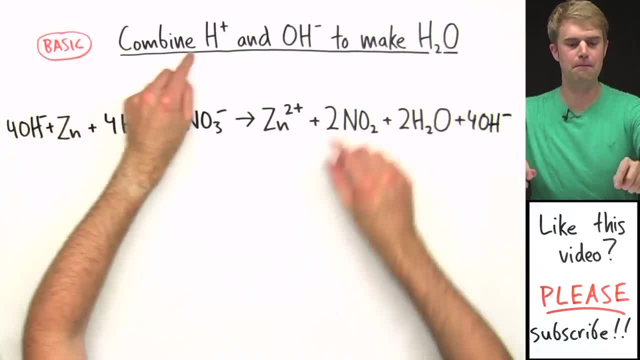 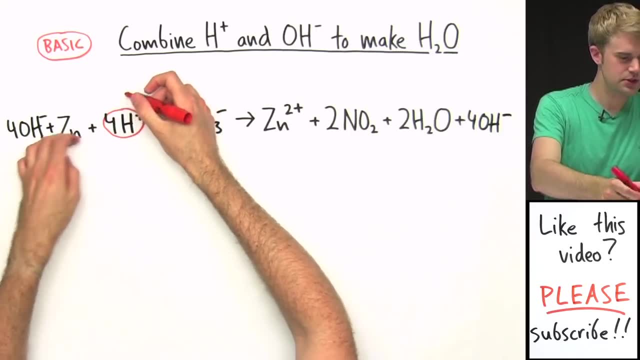 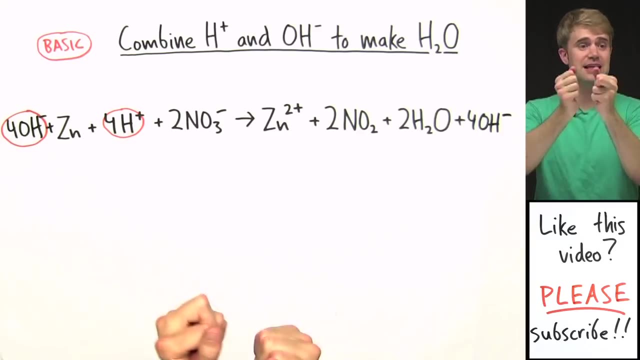 that I'm going to do is I'm going to combine the H plus and OH minus to make H2O. so I have this H plus or these H pluses and these OH minuses. when H pluses and OH minuses come together, they make 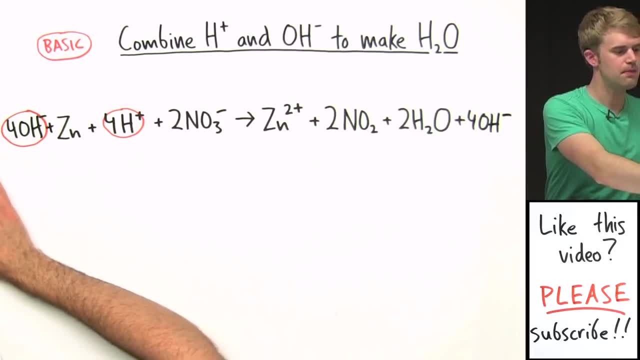 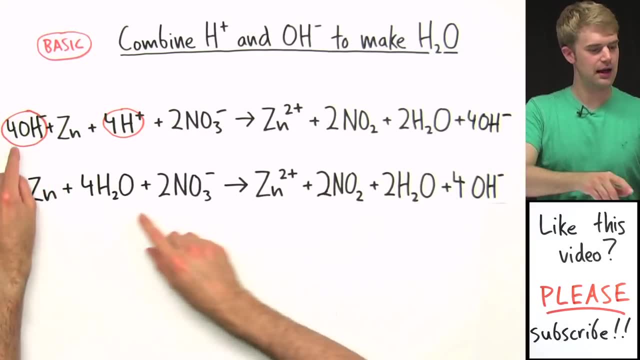 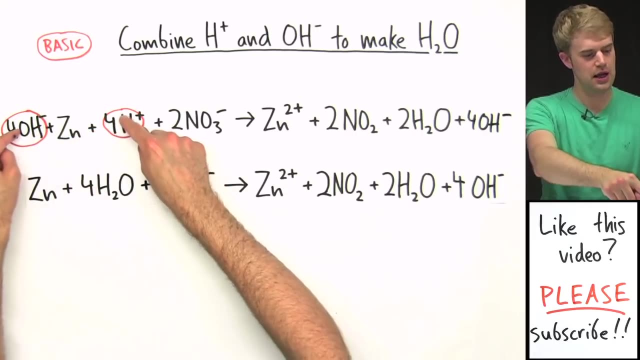 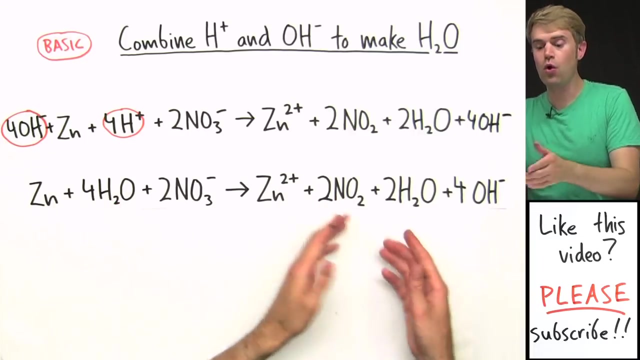 water, okay. so here is the equation that we're going to get when we combine those to make water. you see, on this side I have the four OH and the four H plus, or I should say the four OH minus and the four H plus. they came together to make four H2O. okay, nothing happened on this side because there weren't any H pluses. 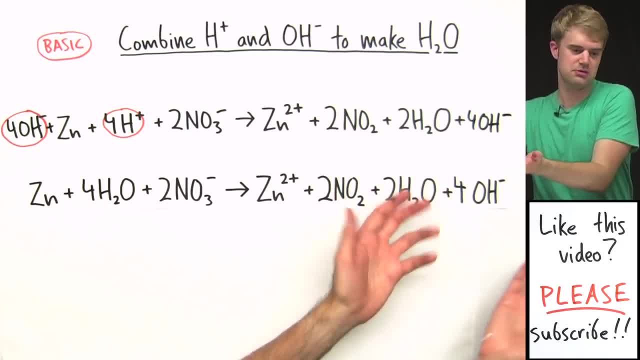 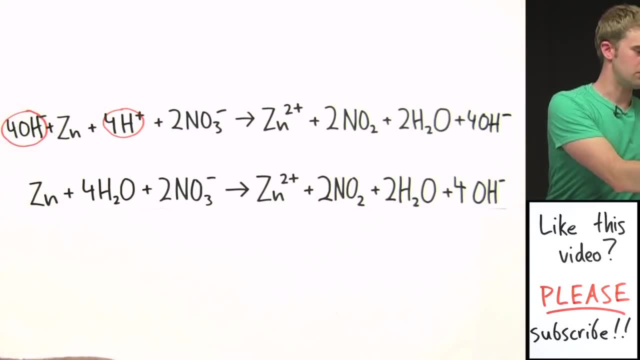 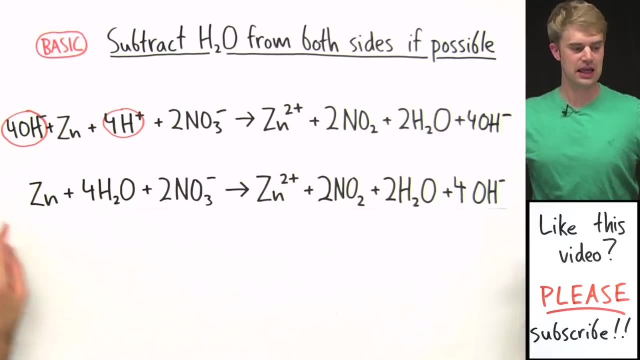 for the OH minus to combine with. so the four OH minus are just sitting over here, okay, so now our last step for basic solution here is that I'm going to subtract that H2O from both sides, if possible. okay, think of this sort of like a math problem. okay, I have H2O. 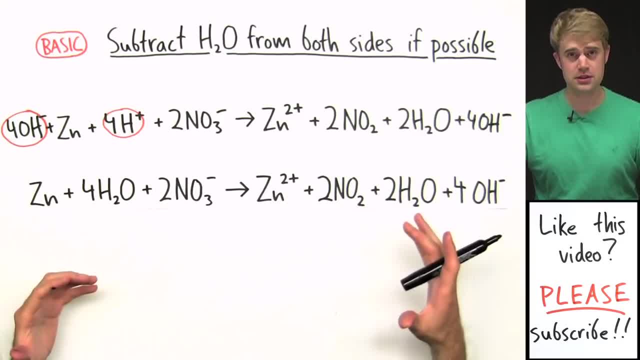 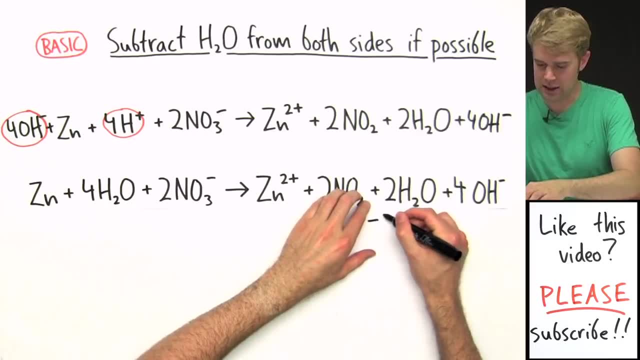 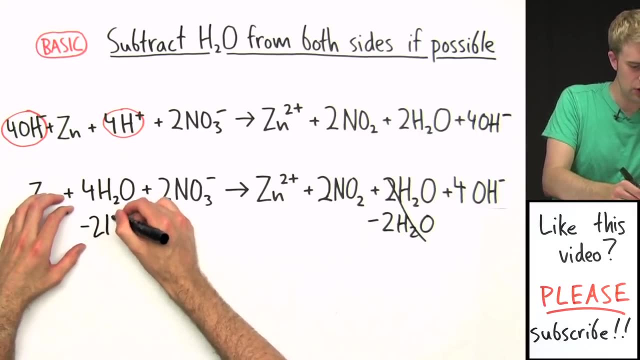 here and I have H2O here, so I can subtract something if it appears on both sides. so I have two H2O here, four there, so I can do minus two H2O and that will cancel that out. I can do minus two H2O and that will leave me with. 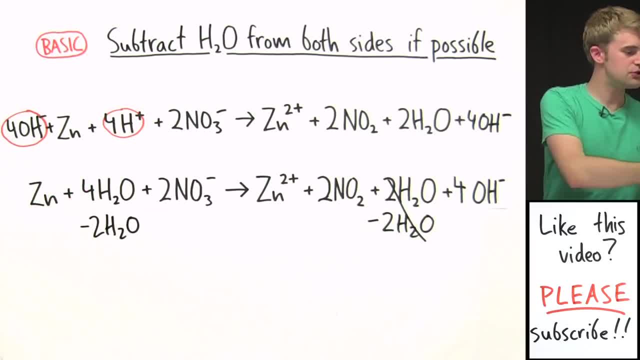 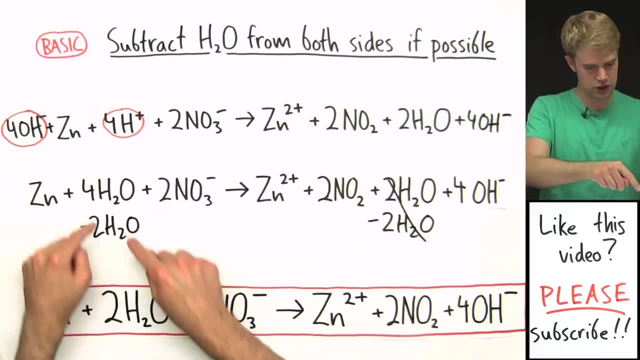 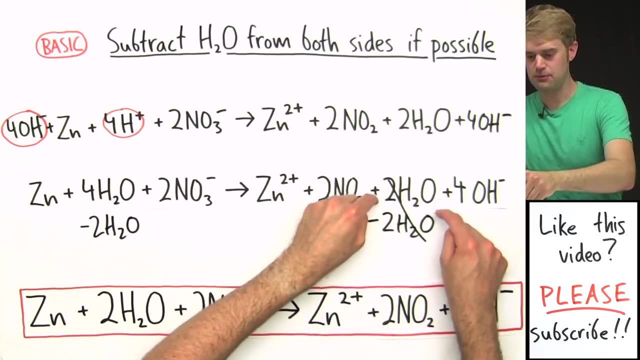 H2O on this side, because 4 minus 2 is 2.. So this will be my final equation: I have zinc plus 2 H2O because I subtracted 2 from here plus 2 NO3. 1 minus gives me zinc 2 plus 2 NO2.. Then I subtracted. 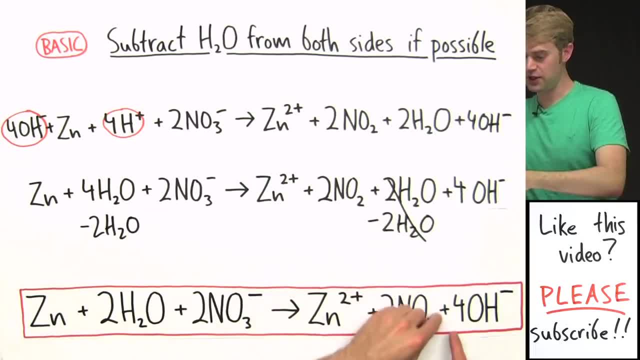 away my water, my H2O from this side. so there's none left, plus 4 OH minus. So I got rid of these H pluses and I'm left with OH minuses. so this is going to be, in basic solution, The last thing that 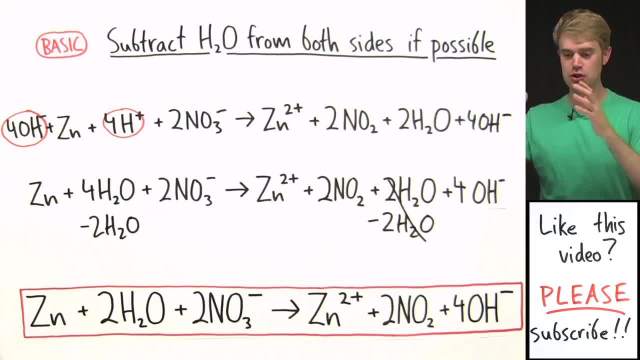 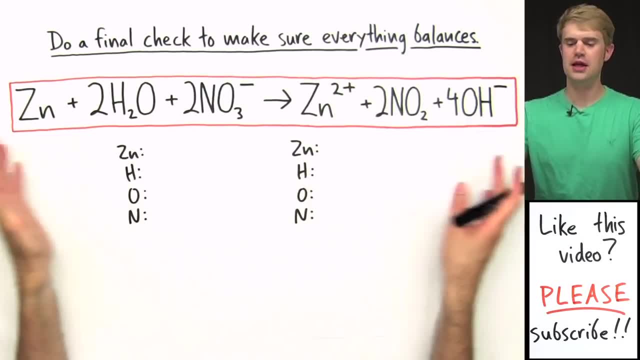 I'm going to do is I'm going to do a final check to make sure that atoms and charge balance, just because I want to have a confidence that I did it correctly. All right, our final check. I discover mistakes all the time when I'm doing a final check of this kind of equation balancing, so I 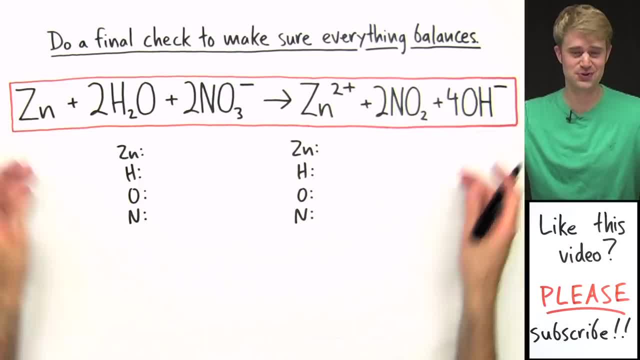 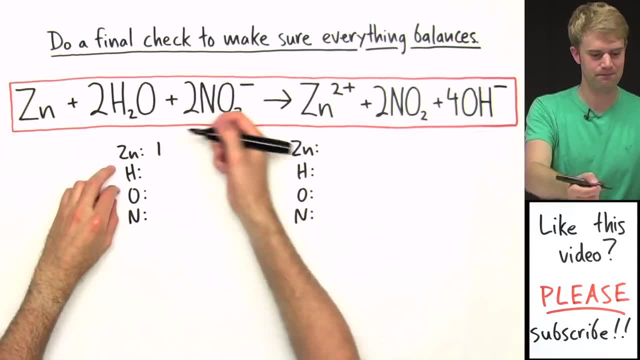 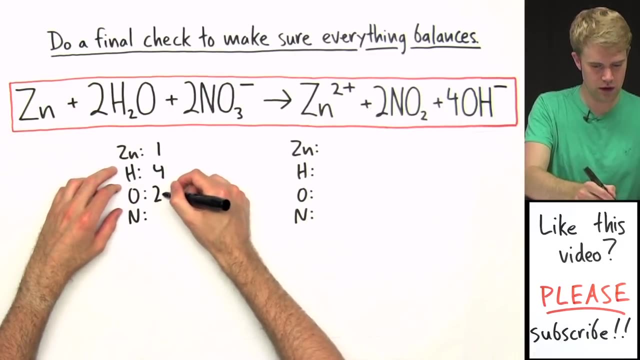 highly recommend that you do this too, just to make sure that your answer is right before you hand in your test or you hand in your homework or whatever. Okay, Zn, we have one of them. Hydrogen 2 times 2 is 4.. Oxygen: I have 2 here, 2 plus 2 times 3. 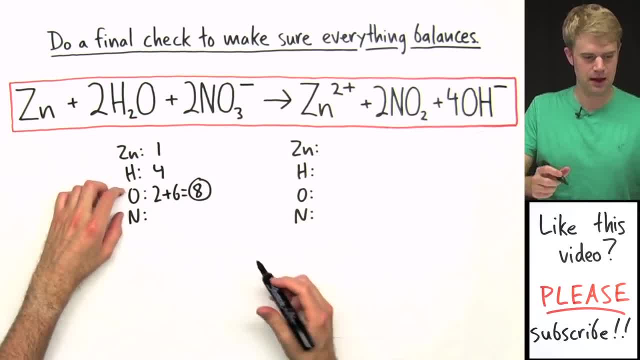 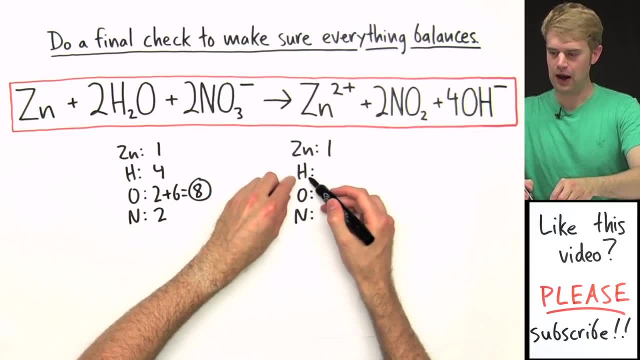 which is 6, gives me 8. and then I have nitrogen. I have two of them. Okay, over on this side zinc, I have one Hydrogen 4 times 1 from the OH minuses, so I got four hydrogens. Oxygen I have two of.